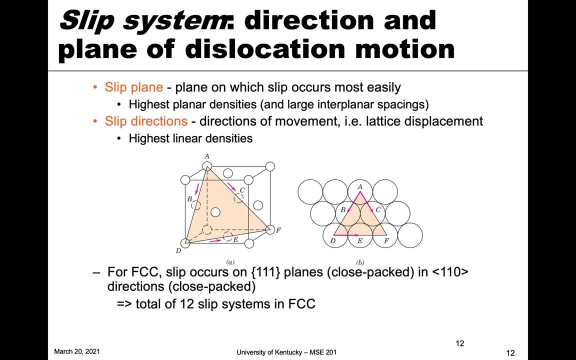 planes within the material, And so those tend to be the ones with large planes, interplanar spacings also along in that plane, slip occurs in a specific direction, and so the slip direction is the direction of movement. so this is that lattice displacement, so this is the direction, with the same direction as the 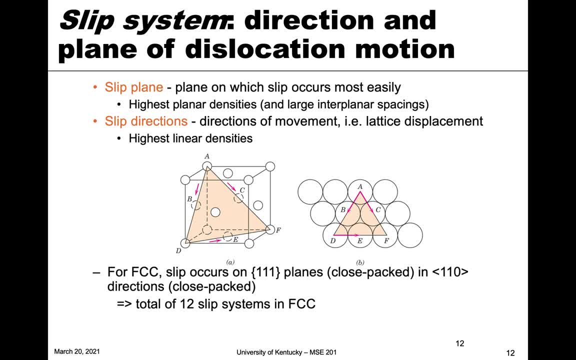 burgers vector. and again easily this: we can kind of define slip directions for the most part as being the directions that have the highest linear densities, and so you know. if you're wondering why we kind of talked about planar and linear densities in the previous chapter, excuse me, this is one of the reasons. 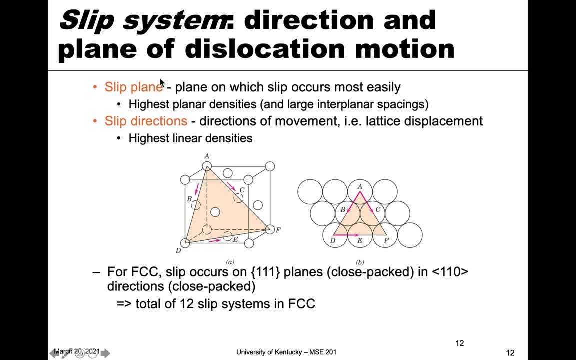 right because it helps us look at what might be a slip plane and slip direction, because it has the highest planar densities, and so here we're looking at, for example, in FCC- this is an FCC crystal- we have the 1, 1, 1 type of plane highlighted and we can see that the 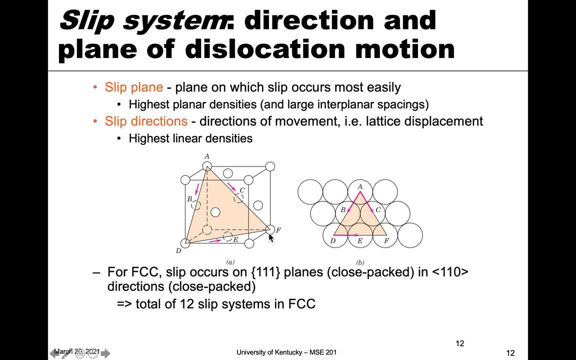 arrows indicate possible motion slip directions. so we have the slip plane highlighted and then possible directions and if we recall from FCC the 1 1: 1 plane was the close packed plane and we can see from this diagram of the 1 1: 1 plane that the edges of the triangle here occur on a 1 1: 0 type. 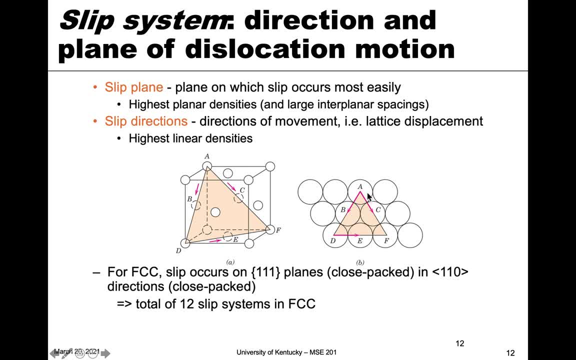 direction, which are also the close packed directions, because that's where those atoms are in close contact. so if we kind of take for this FCC a, That we could have any of these 1, 1, 1 type of planes, because they're all equivalent. 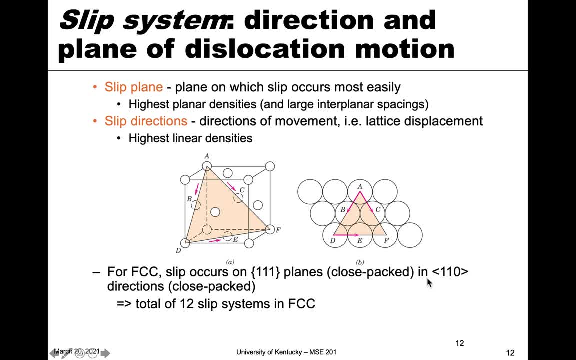 And same thing with the 1, 1, 0 direction. Those are all equivalent as well. It gives us a possible combination between those of 12 different slip systems, So it's 12 different combinations of plane and direction, And that means that in FCC we have 12 possible slip systems for motion of a dislocation to occur. 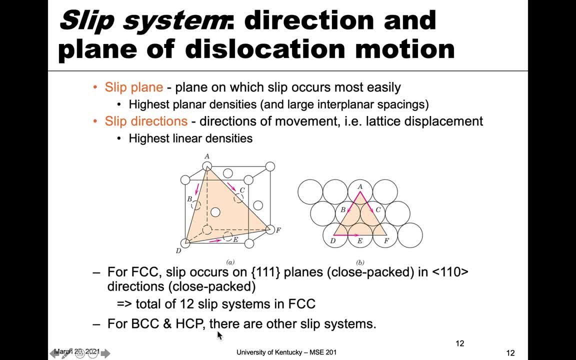 For BCC and FCC. there are other slip systems, right, But it tends to go by the highest planar and linear densities, for planes and directions respectively, And so let's look at some examples then. So here in this table, which is also in your textbook, 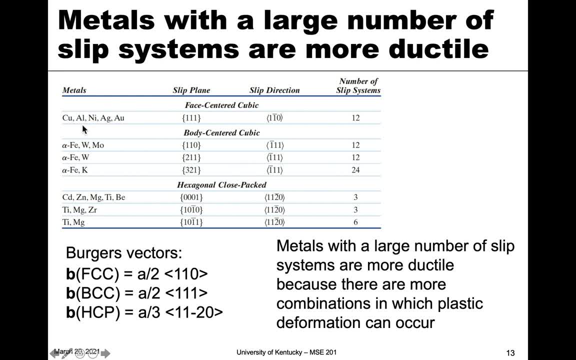 you see that For FCC metals- so copper, aluminum, nickel, silver, gold are all examples of FCC or face inner cubic metals, And so their slip planes tend to be again 1,, 1,, 1. And this means family of planes. 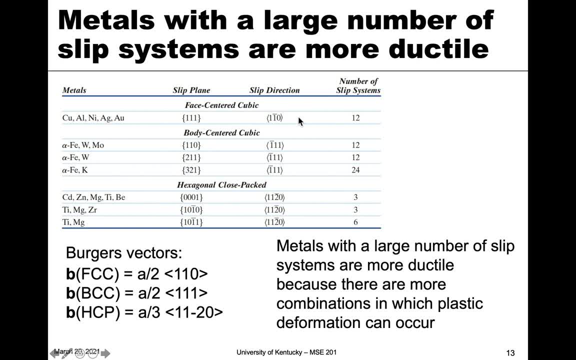 So it could be any one of the 1, 1, 1 type, And we can also have a slip direction of the type 1, bar, 1, 0. And again the combination. You have 12. Things get more complicated for BCC and HCP. 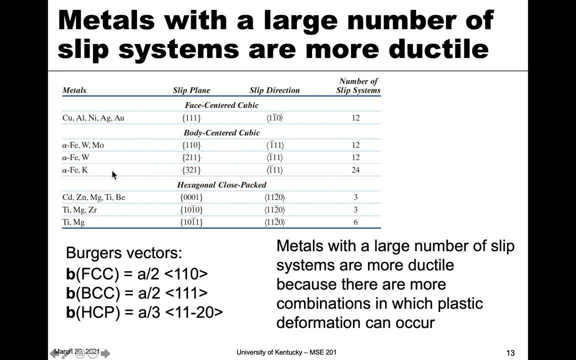 in that for different metals you can actually have different slip systems. So for alpha iron, tungsten and molybdenum we tend to have the 1, 1, 0 plane and the bar 1, 1, 1 direction. 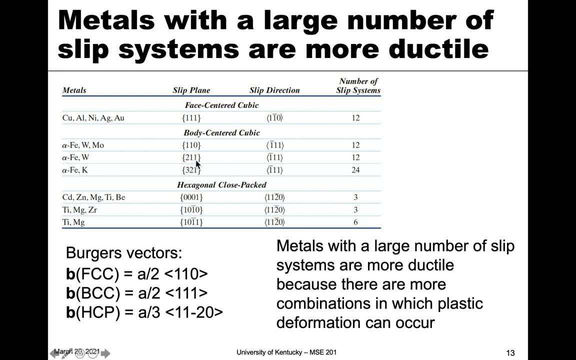 Whereas you can also have the 2, 1, 1 and the 3, 2, 1. As possible, planes with a similar direction. So the directions don't change, but you can have different cases of slip planes, And the same thing can be true of hexagonal close-packed. 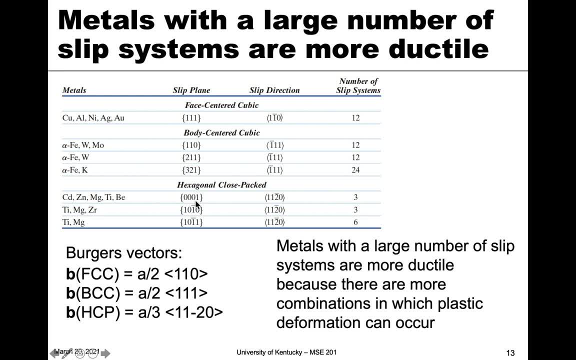 They tend to be the close-packed, so the basal plane, which is the 0, 0,, 0, 1.. But you can also have others in certain instances, And then the directions are those close-packed directions, which is the 1, 1, bar 2, 0.. 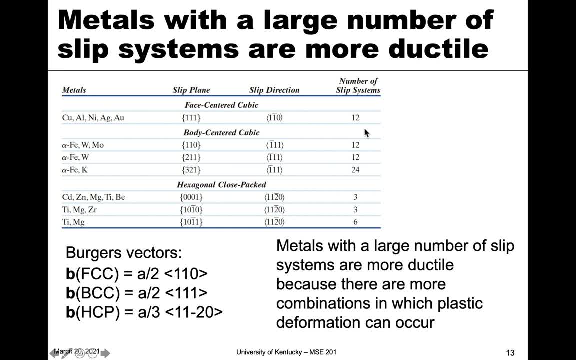 And with those you tend to have fewer or the same slip system. So BCC has 12 and 24 in certain cases, But HCP has less of these close-packed directions because there are less basal planes in HCP than there is in FCC. 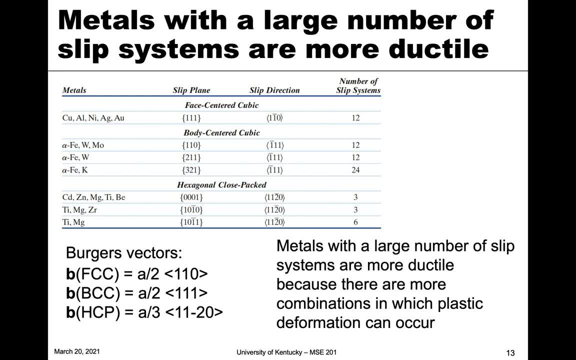 where there's a number of these close-packed planes, The Berger's vector also will be a fraction of the slip direction And in each case it's either the lattice parameter divided by 2, divided by 2, or divided by 3.. 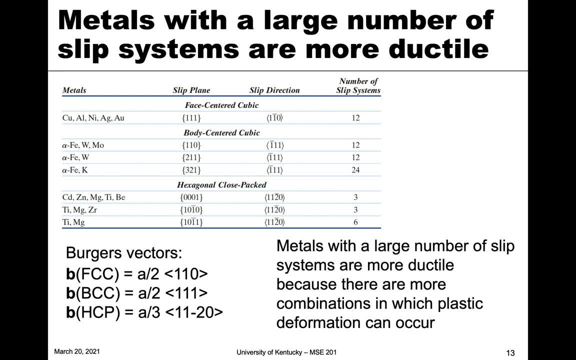 And that's the magnitude of deformation that occurs. So each motion or step that occurs, that's what the Berger's vector is here, And the general trend we see with this is that metals that have a large number of slip systems tend to be more ductile. 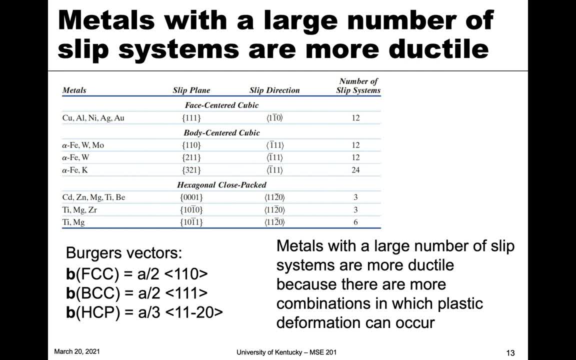 They end up having more plastic deformation, so they're more ductile Because there's more combinations in which plastic deformation can occur. So FCC metals- and you probably have an idea of these- copper, aluminum, nickel, the noble metals like silver and gold, right. 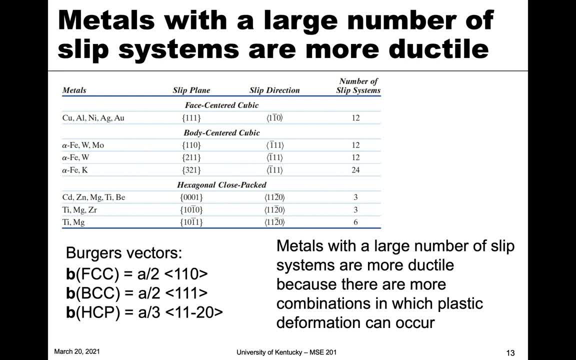 Those are very ductile. Right, Those are very ductile metals that can be hammered into shape very easily, However, something like an HCP metal, like titanium or zinc or cadmium or magnesium. those are relatively more brittle because there's not as many combinations of slip systems. 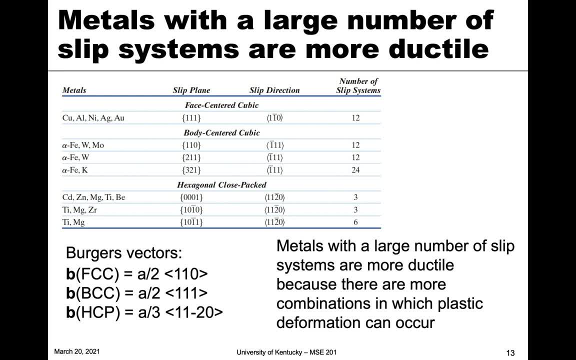 And so HCP metals tend to be more brittle, And so we can get that by looking at the combination of slip systems available for those particular metals. And so we can get that by looking at the combination of slip systems available for those particular metals.